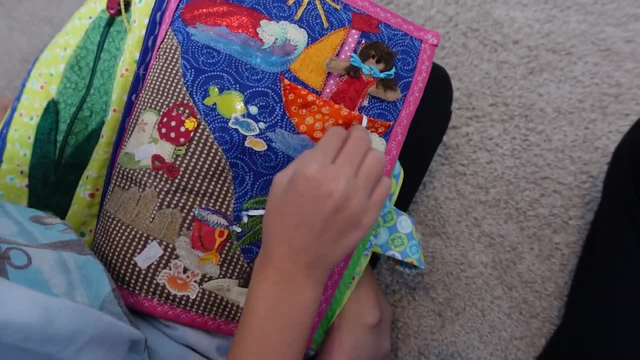 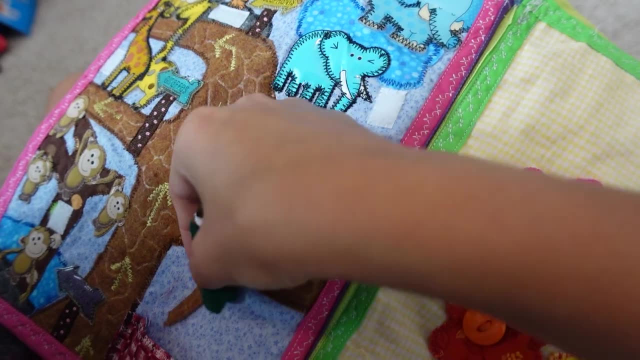 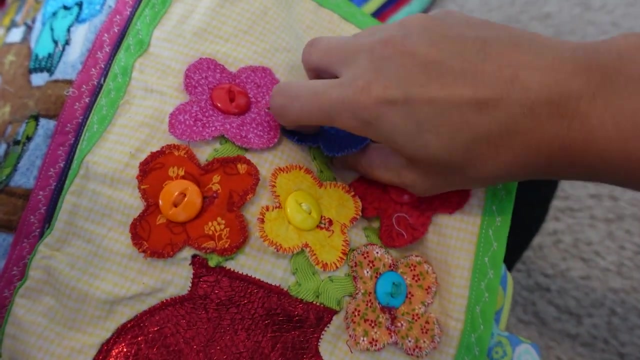 Plus, if you're creative and good at sewing, this would be such an awesome project to do yourself or your own kids or as a gift. This first book that I'm showing you is Riley's, and obviously that's the first one my mom made, because Riley is my firstborn. I know when she started out she got a lot of ideas from Pinterest and then she just sort of started doing her own thing. 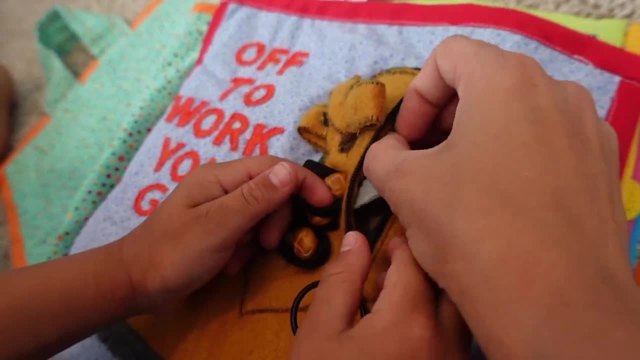 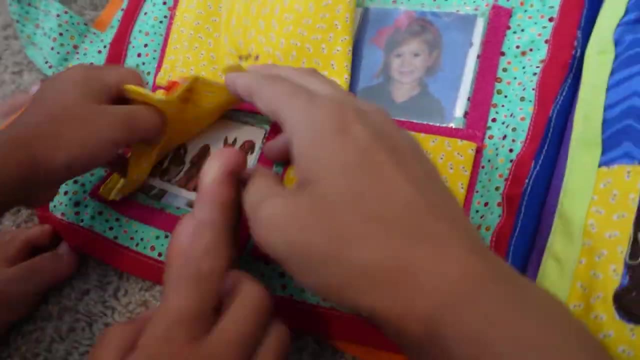 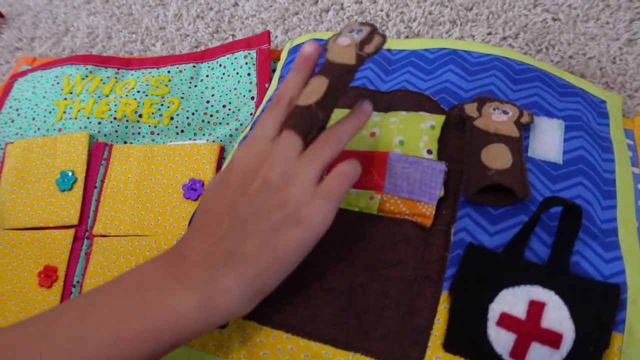 These books are so cute and fun and educational. The kids have a blast with them. Watch them interacting and singing along to this monkey. on the bed page, for instance, There are a lot of monkeys jumping on the bed. One fell off and hit his head. 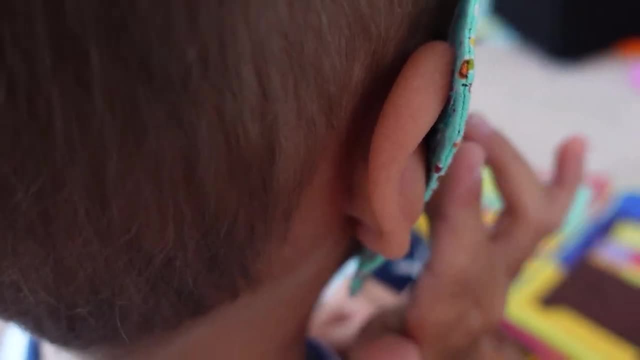 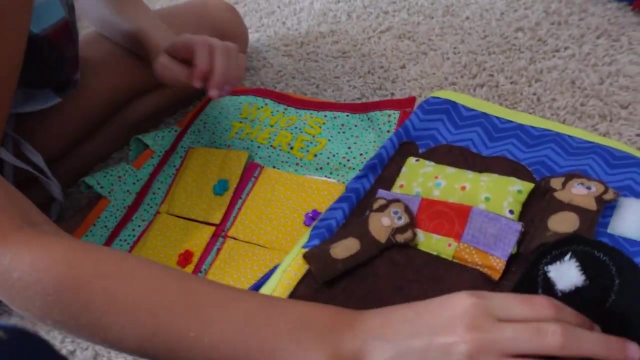 Now you're going to call the doctor. Mommy called the doctor and the doctor said: no more monkeys jumping on the bed. Alright, now give him his band-aid. Now, where are we going to put it? Let's put it here. 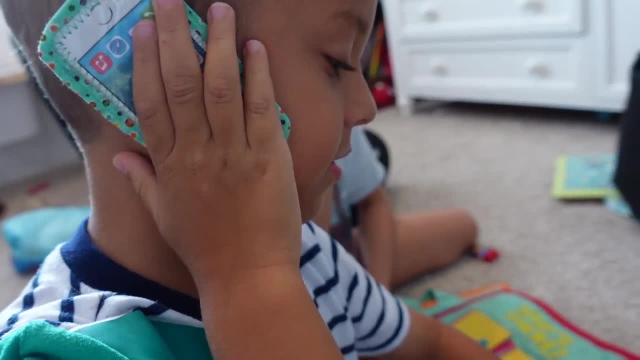 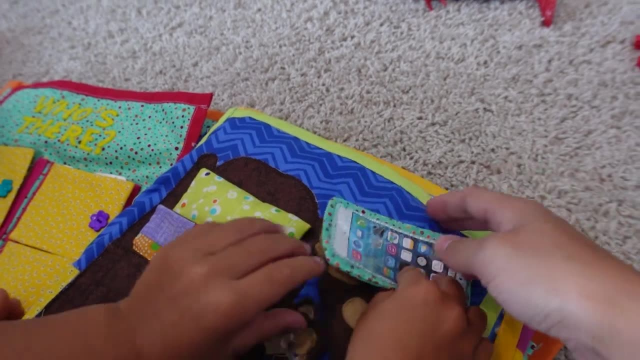 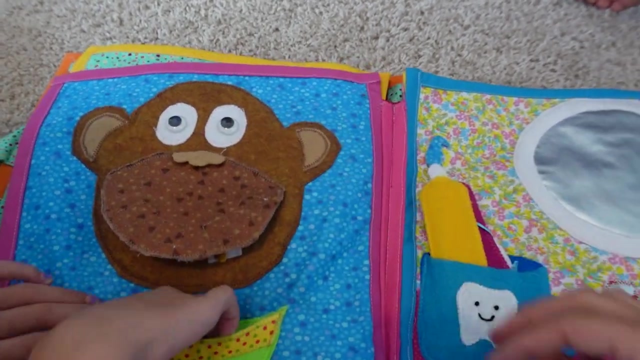 It's on his head. The doctor said: no more monkeys jumping on the bed. Alright, hold him, Give him his band-aid. Good job, Ow, he hurt his butt. Let's show this fancy iPhone. You have to admit that was pretty cute, even with the noisy baby in the background. 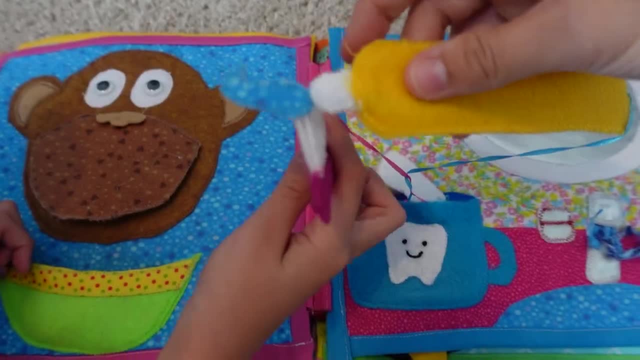 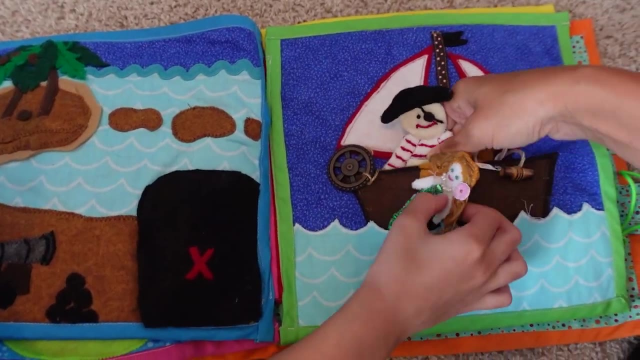 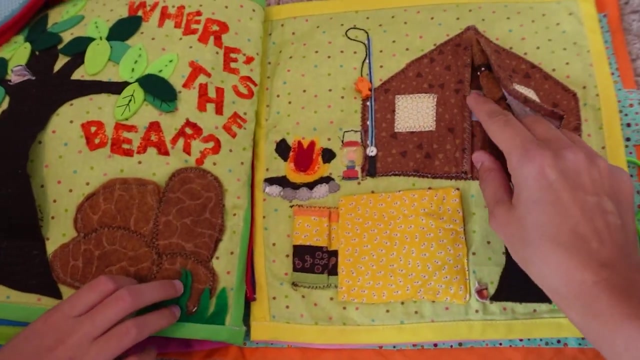 I had to very much fight the urge to show you every single page and how amazing and inventive every single one is. But I had to contain my urge and just show you some of my favorite pages, Like this pirate one with the treasure map that you follow and it leads you to treasure. 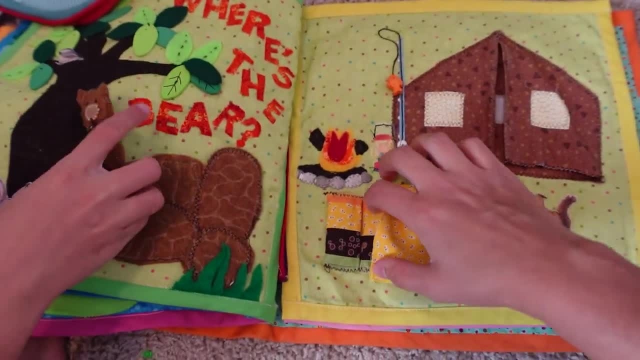 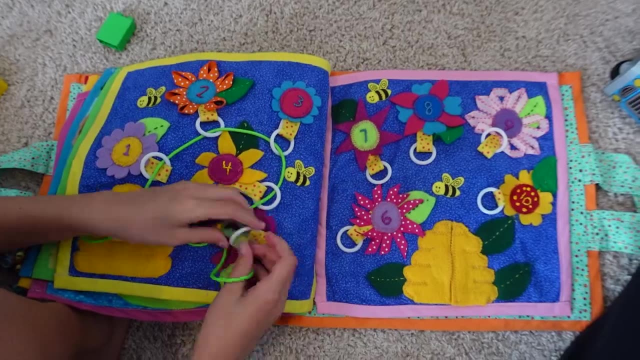 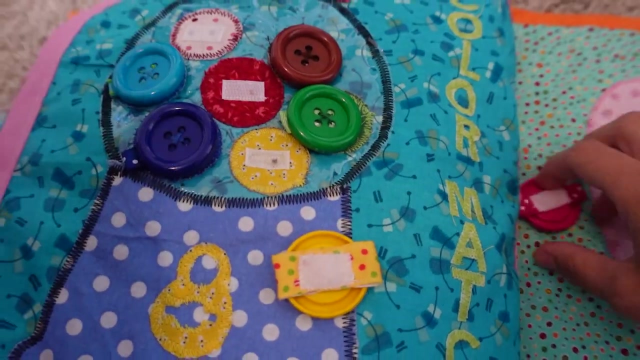 Or this: where's the bear page, which is an adorable little peekaboo hiding game, and I can hide the bear and I can guess where it is. There's counting puzzles, color matching, lacing, buttons, zippers and loads of pages that are just perfect for creative play. 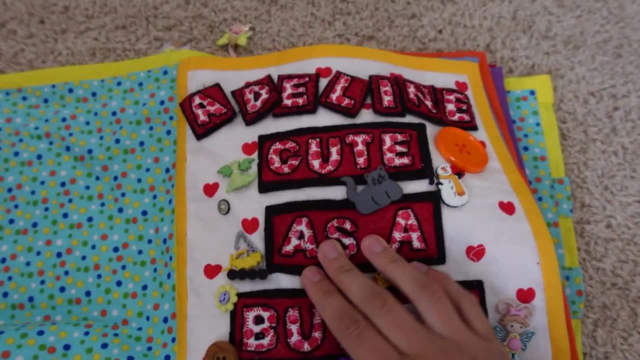 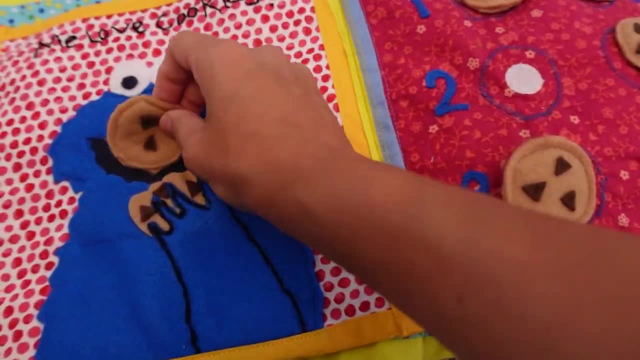 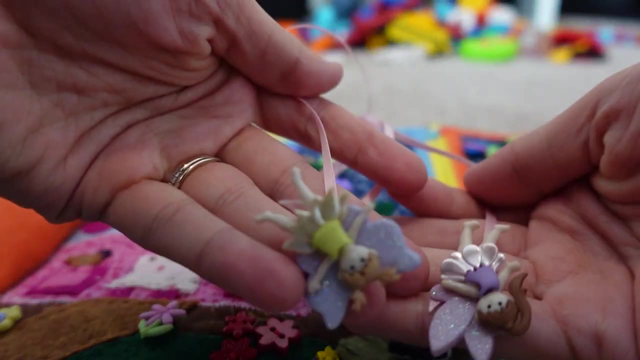 This third book is the last one. This is Addie's little book, And while I know that she's still too little to fully enjoy them- right now- she's only one year old- I plan on treasuring these forever. I truly hope that they pass them on from generation to generation like a family heirloom. 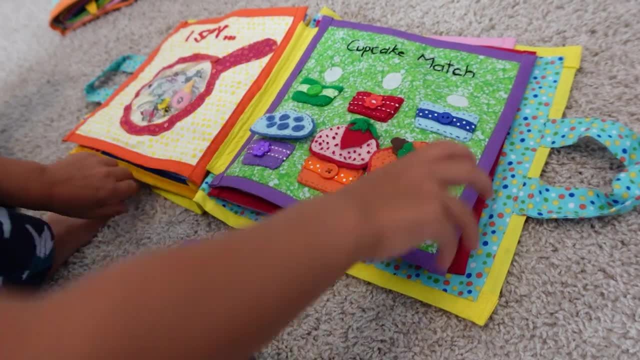 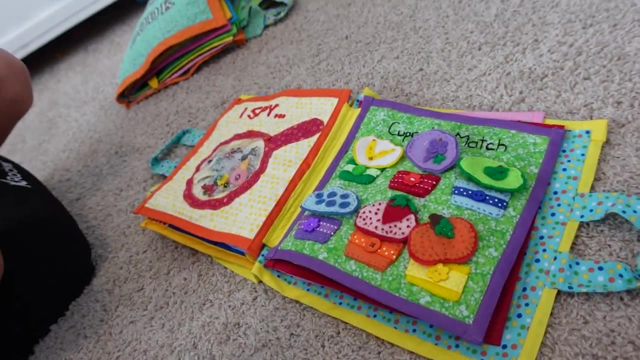 Even this simple little color matching cupcake game. it's so cute how they can be creative with how they play with it. For instance, Holden used this to kind of mix up the colors and be funny, And then, of course, you can use the right way. 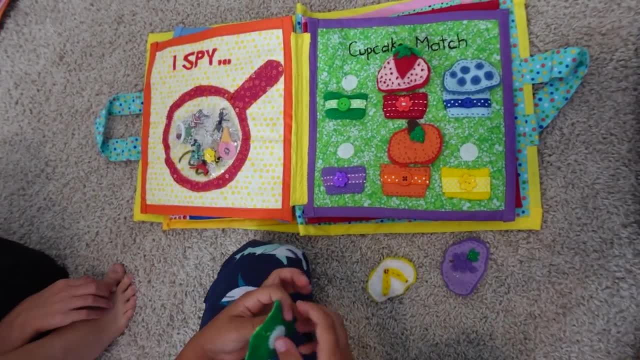 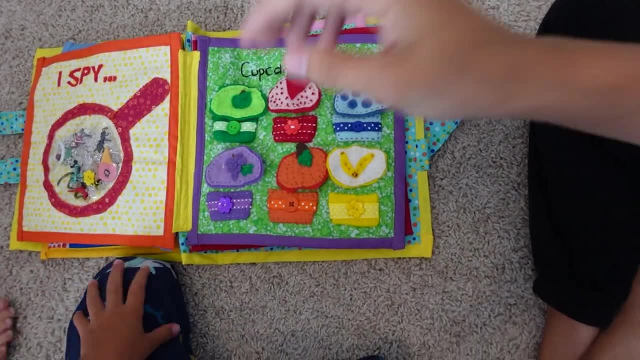 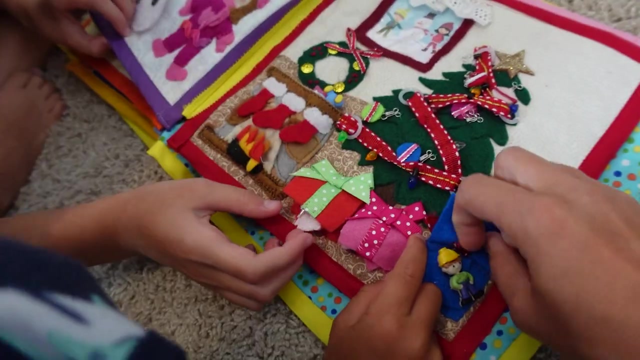 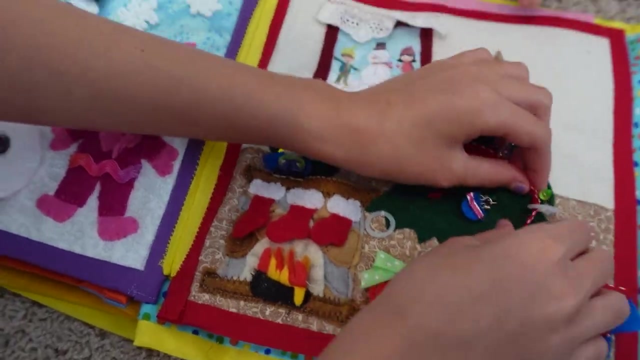 But it's so cute to watch kids' minds working and their gears turning. Sometimes they can take something so simple and make it so unexpected and fun. I really wanted to show you this particular page. The detail in this is insane. The snowman comes together like a puzzle and then the presents under the tree are interchangeable with other pieces in the fireplace. 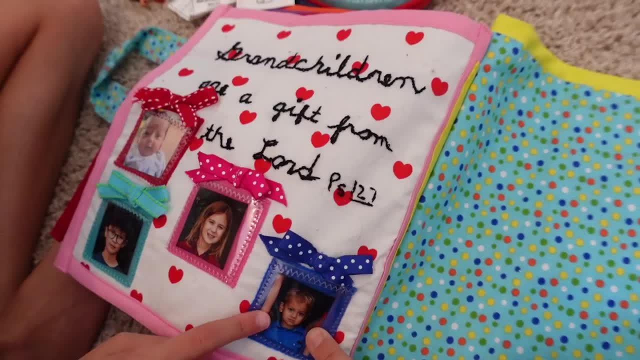 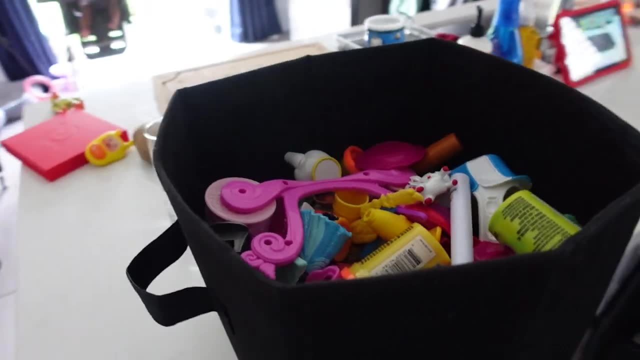 And then the garland on the tree is lacing. Amazing. That's Holden, that's me, that's baby Addie and that's our cousin. Our next activity is a classic: It's Play-Doh. I love Play-Doh. 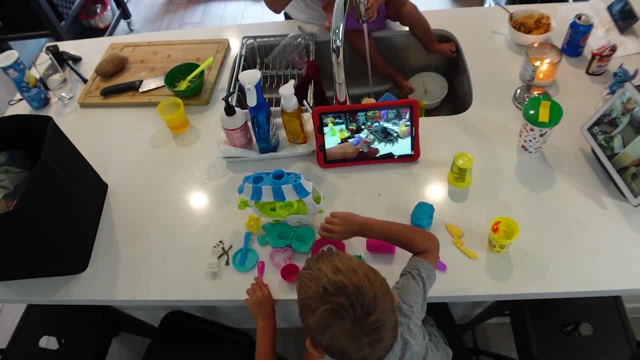 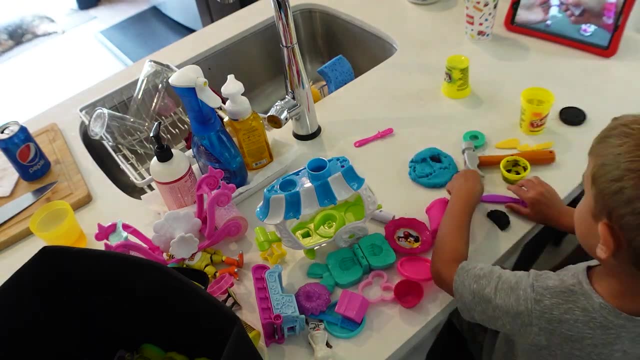 I know some people hate Play-Doh, mostly because the cleanup stinks. But stick around because I have a really good tip and another activity that's really fun to clean up when you're done. Play-Doh is one of my favorite ways to get tactile and hands-on. 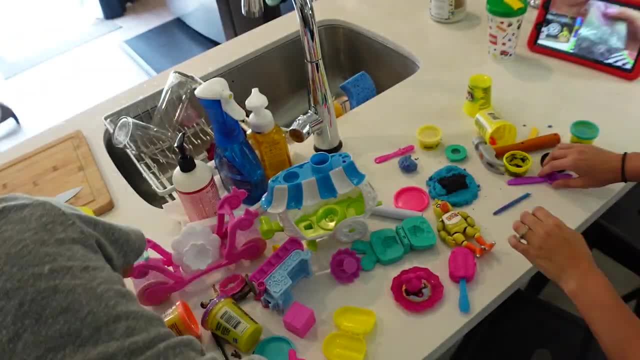 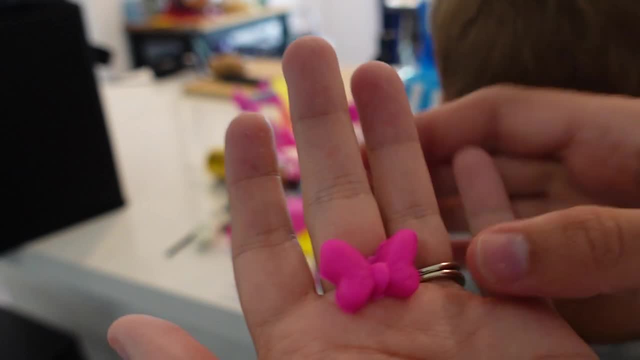 You can build and model so many things, And they have all kinds of toys to engage your child in, whatever interests them, whatever character, whatever it may be. For instance, Holden is really into Five Nights at Freddy's right now. So we decided to make Chica some accessories, starting with this bow. 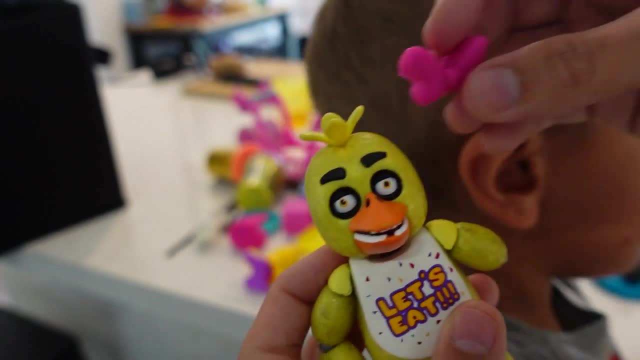 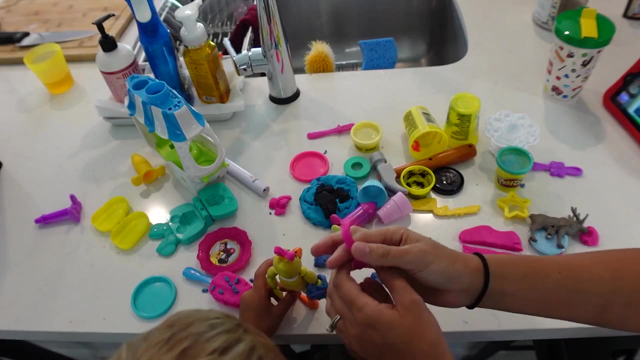 Even if you don't have any fancy Play-Doh toys with molds, you can use whatever you have on hand: Toys, kitchen utensils, things that you find outside. You can even make your own Play-Doh, which we've done quite a few times. 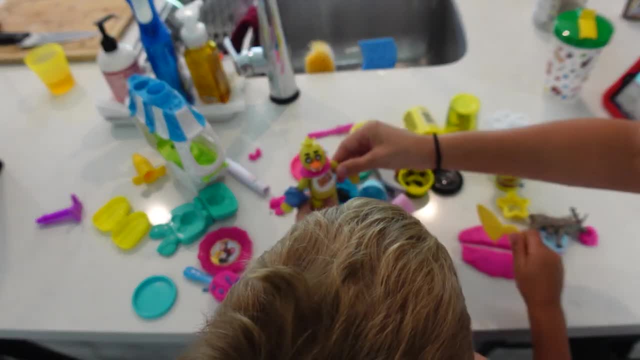 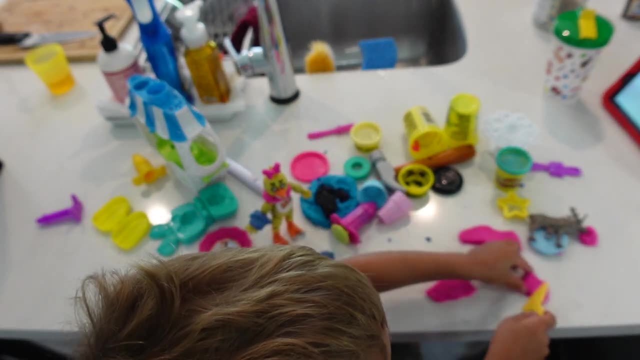 It's a really simple recipe and the kids can help. They can add color or scents and make it their own. Playing with Play-Doh encourages more than just creativity: It also helps improve hand-eye coordination and work on those fine motor skills. 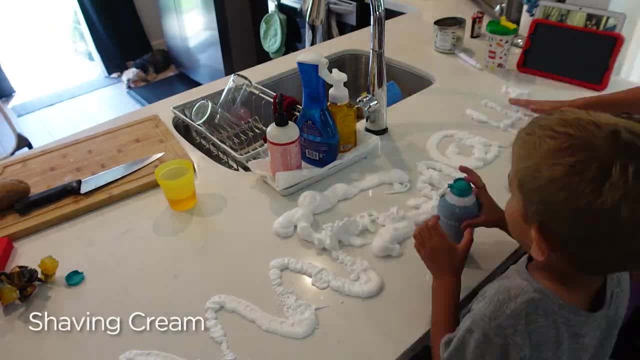 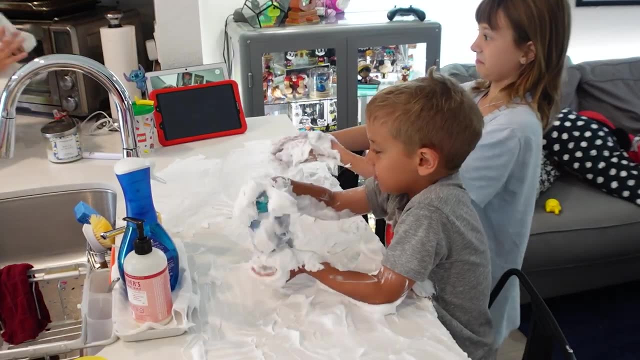 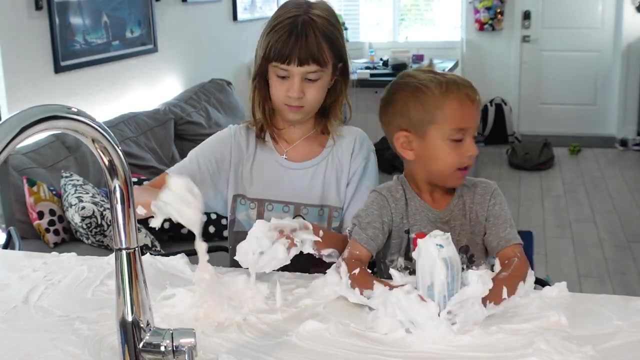 Here's my creative idea for cleaning up the Play-Doh and having another fun educational activity the kids can enjoy. After we tidied up the Play-Doh, we went crazy having fun with shaving cream on our counters. You can use it to write letters and draw pictures, or play with toys or just get messy. 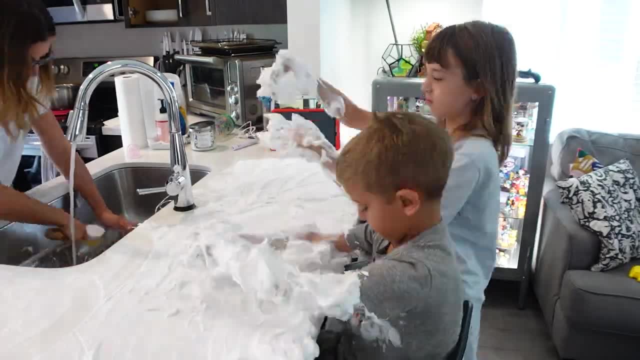 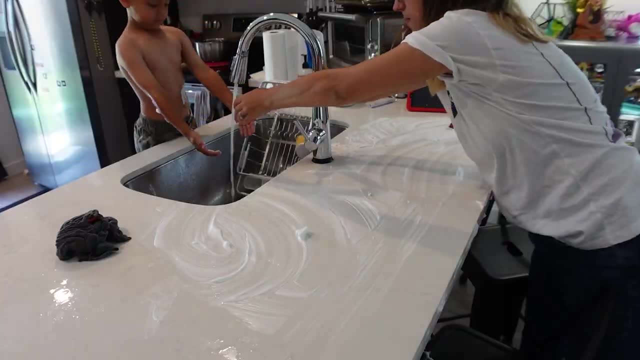 We've done something similar in the past. We made shaving cream cupcakes in a sensory bin in the backyard, But using it to clean my counters was a stroke of genius. I was surprised how long this kept them busy, And the best part is that it smells really good when you're done. 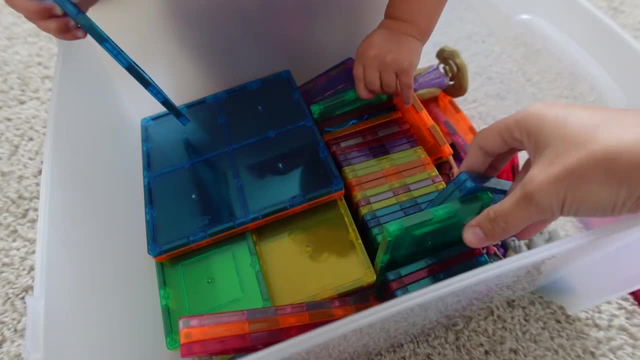 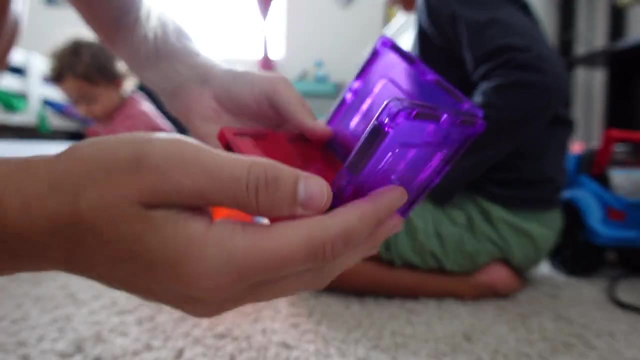 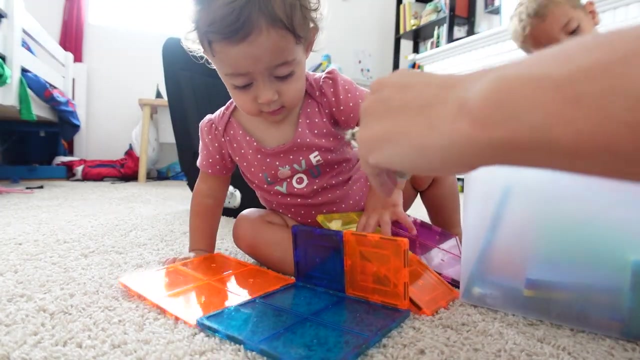 And it left my counters sparkly clean. The last activity is these magnetiles, or magnetic blocks. My kids love these and they can play with them for hours. They have these magnets on the inside corners so they attach to one another. They're an open-ended stem toy that you can use for creative, imaginative play. 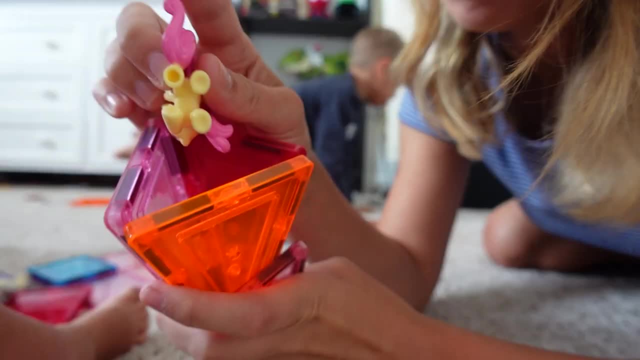 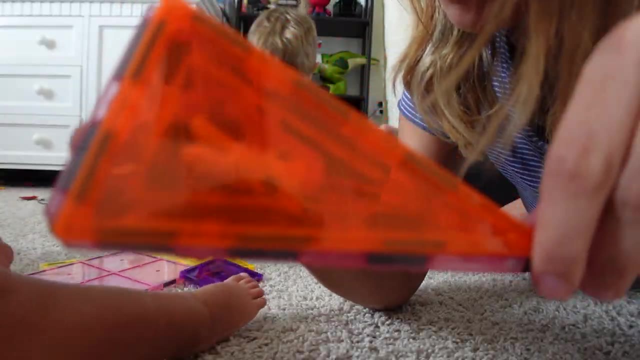 Teaching colors, shapes, engineering, gravity and, of course, magnets. My kids particularly like putting their toys inside of them like a blind box and then being surprised, Or building prisons to trap their toys Or making gigantic structures that are a blind box. 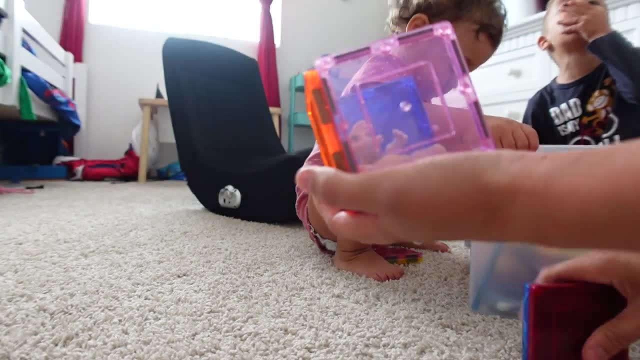 Or structures that are a blast to destroy and knock down. Eat them. And then I went. 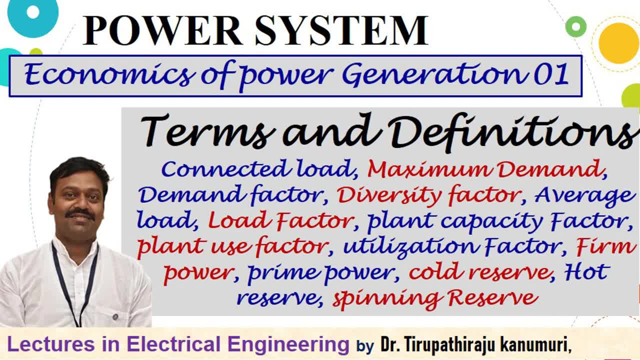 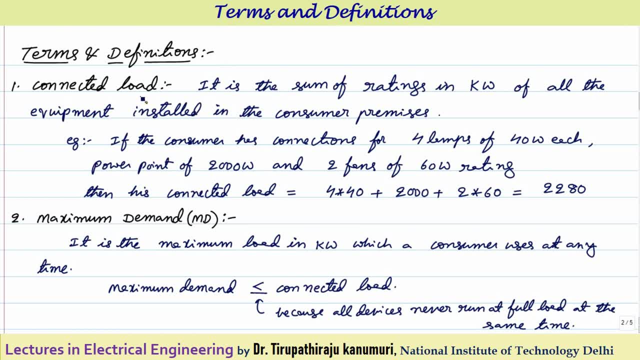 Hi all. today we are going to discuss different terms and definitions related to economics of power generation. So let us start the terms one by one. First one is the connected load. So the name itself is telling: connected load. that means the total load that is connected is called as the. 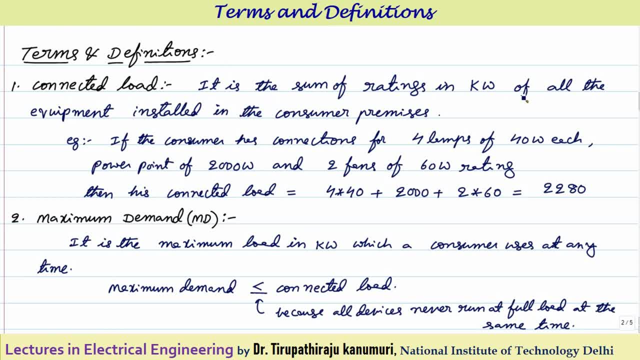 connected load. Actually, it is a sum of ratings in kilowatt of all the equipment installed in the consumer premises. Let us take, for example, I have my house. So in my house, a small house, I have provided these following things: I have provided four ports. that means four lamps of 40 watts each. 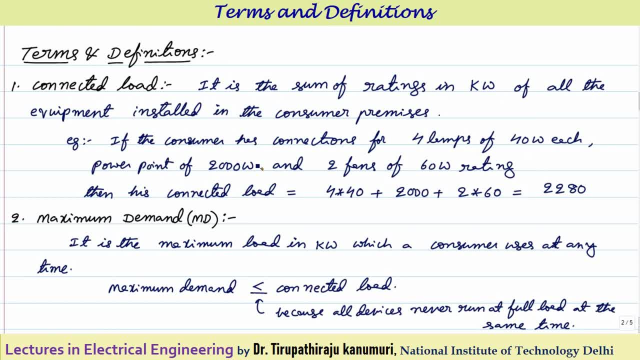 and I have provided a power plug of 2000 watts, only one plug, and I provided two fans of 60 watt rating. So I may or may not use all these equipment, but these are installed in my house. These are the different ports that are available in my house, So that is called as the connected load, So that